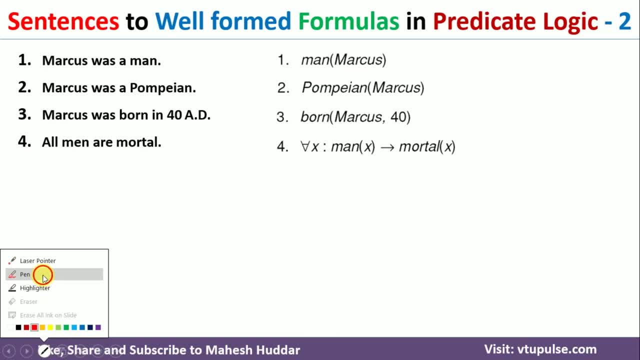 men and that is for all x. If x is a man, then x is a mortal over here. So that is a very simple statement again over here. Coming back to the next one, all Pompeians died when volcano erupted in 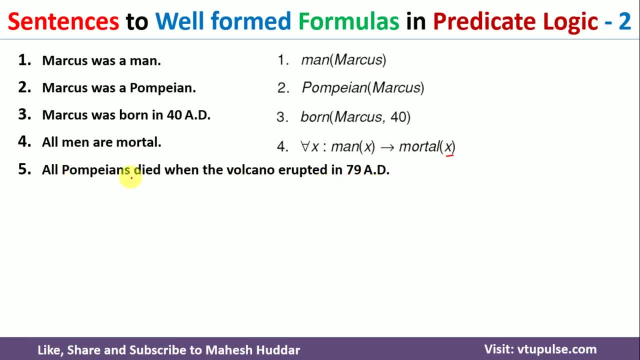 79 AD. So all Pompeians that's nothing but if x is a Pompeian, then x has died in 79 AD. So that is the first thing. At the same time, there is one more thing has happened that is volcano erupted. 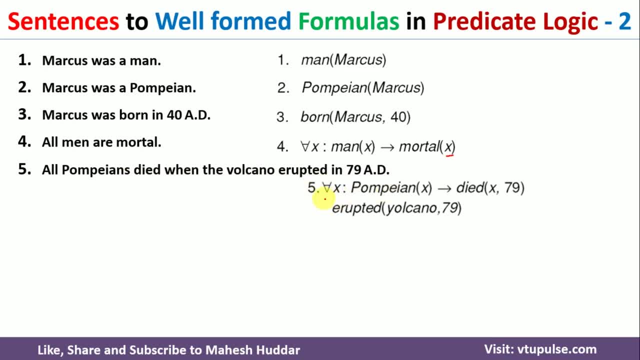 In this case, so this can be represented something like this. For all x, if x is a Pompeian, then x has died in 79 AD. At the same time, volcanoes erupted. So that's the reason we 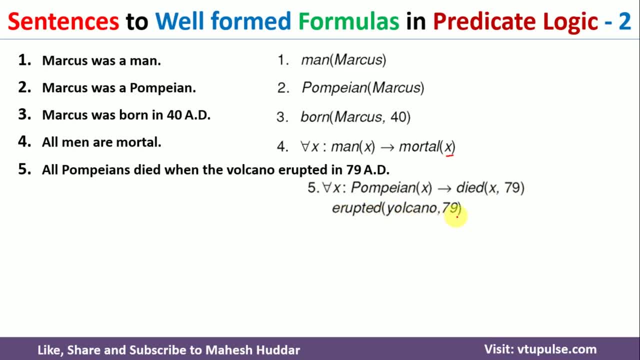 can write something like this one erupted volcano comma 79 over here. Coming back to the next one, 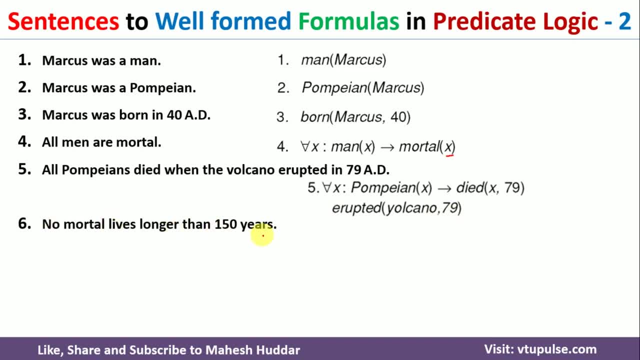 no mortal lives longer than 150 years. So in this case, we have to do some comparison here. Let us say that the mortal has born, at a time t1. And the current time t2 is greater than you can say that it is more than 150 years 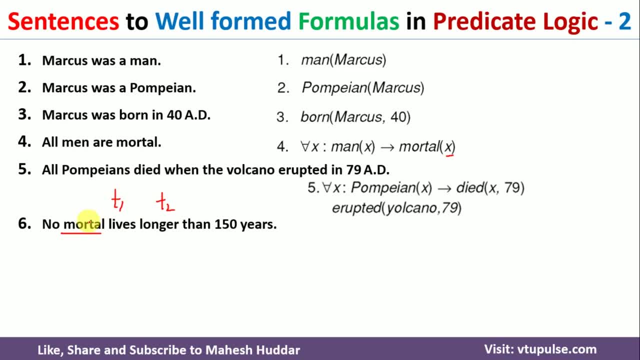 compared to t1. In that case, the mortal is not living, it is a dead over here. So what we can do over here is we can take something like this. For all x, for all t1, for all t2. If x is a mortal, 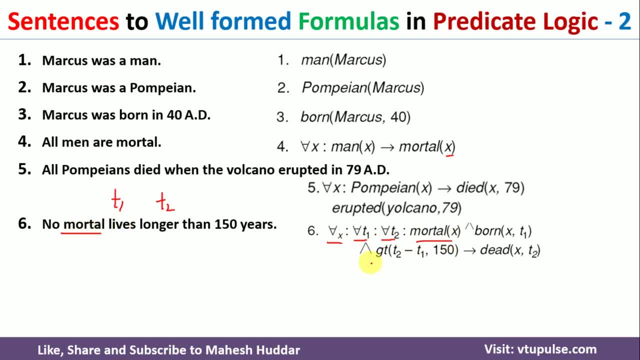 first of all, the x should be mortal. That's the first and foremost condition. And x has born at particular x has born at time t1 that x has born. And this t2 minus t1 that is t2 is 150 years more than t1. That is nothing but what t2 minus t1 is greater than 150. If it is greater than 150, the meaning is at time t2, x is died. So that is what the simple statement over here. 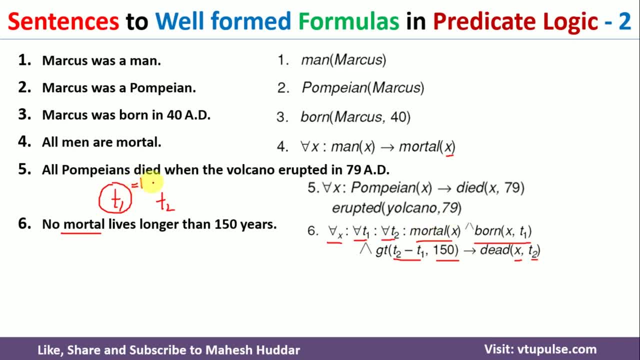 For your understanding purpose, I can take something like this one. Let us assume that 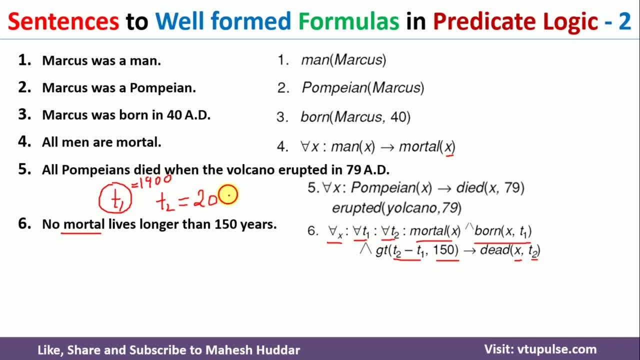 t2 is equal to you can say that 2060 years. Now, if you see here, t2 is 160 years more than t1. So the mortal has born at 1900. And t2, the current year is more than 160 years. Because it is more than 160 years that the x has, you can say that died here. Because after 150 years, that particular 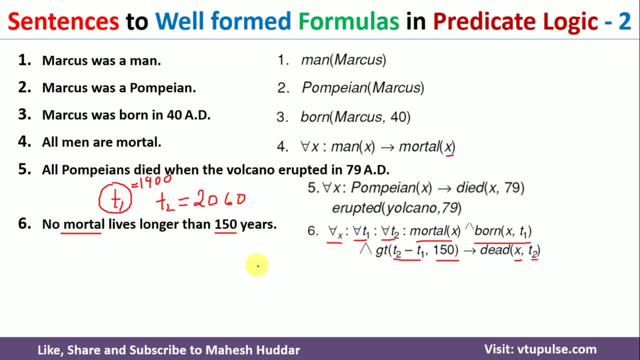 person or a mortal will die here. So that's it. Coming back to the next one, that is, it is now 21. It is a state for Rodan now is equal to 1991 over here. The eighth one is something like this 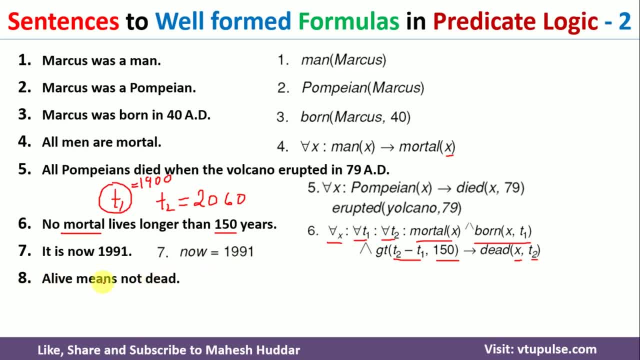 alive means not dead. So it is something like if x is alive, then x is not dead. If x is not dead, then x is alive. That is as simple as that. So that can be represented something like this one, if x for all x for all t, if x is alive at time t, the meaning is x is not dead at time t over here at the same time. And if x is alive, then x is alive at time t. And if x is dead, then x is alive at not dead at time t then x is not alive at time t over here so it's a very simple or straightforward the logical statement over here coming back to the last one that is if someone dies then he is dead at all later times so let us assume that a particular person has died at time t1 the meaning of this one is after t1 i can say that t1 plus 1 t1 plus 2 and so on the particular person is died over here so what you can do here is for all x for all t1 for all t2 if x is died 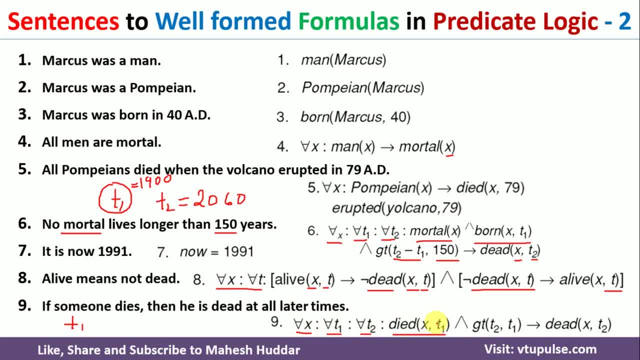 at time t1 so currently the x has died at time t1 and t2 any time greater than this particular the t1 that is t2 is greater than t1 the meaning is what the x has died at that particular time also for example t1 is 1900 okay t2 is you can say that 1901 also ','